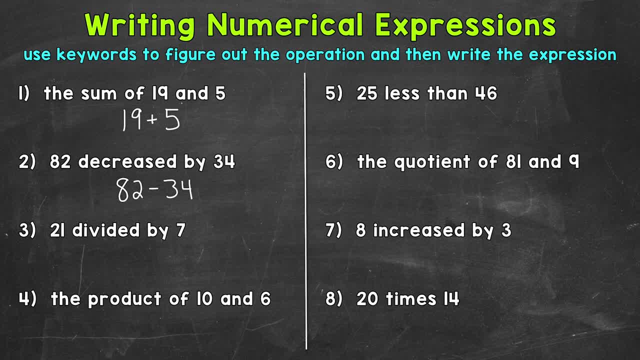 On to number three, where we have twenty-one divided by seven. So here we have division, So twenty-one divided by seven. Now there are different ways to represent division, So that's one way. Another way would be writing it as a fraction. 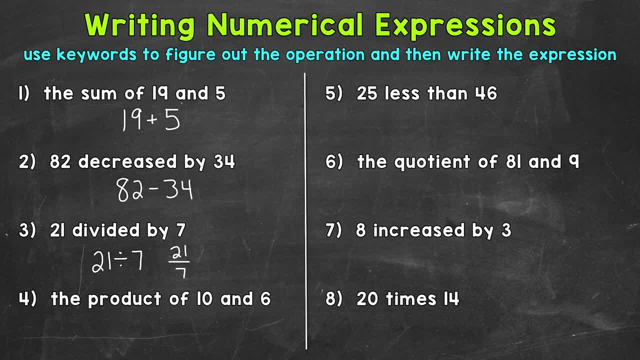 So twenty-one divided by seven. And we can also use a slash, So twenty-one divided by seven. So a few different ways there to represent division. Number four: the product of ten and six, So product. that's the answer to a multiplication problem. 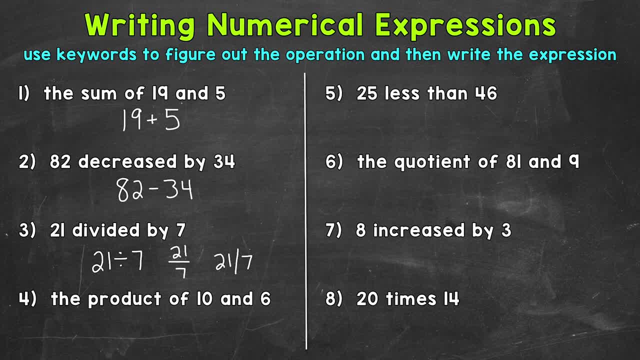 So this is going to be multiplication. So ten times six. So we can write ten times six. We can also use a filled in circle or dot here: Ten times six. We can use an adjective, We can use an asterisk. So ten times six. 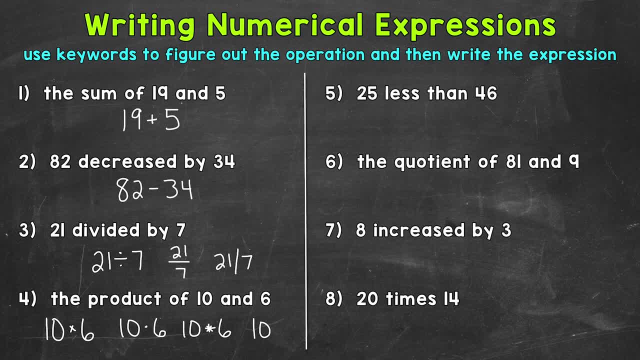 And then also we can use parentheses, So ten times six. So different ways to represent multiplication for number four there. And let's move on to number five, where we have twenty-five less than forty-six. So when we see less than, we actually switch the order. 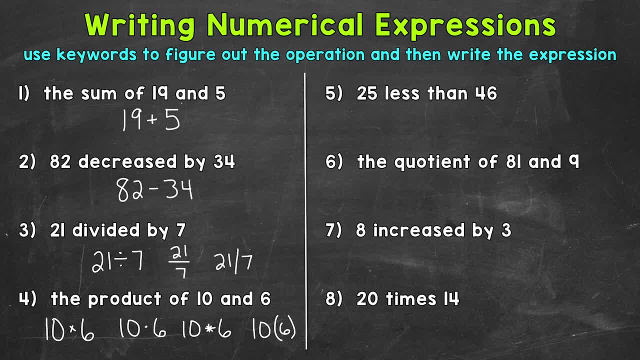 This is going to be subtraction. We're taking twenty-five less than forty-six, So it's going to be forty-six minus twenty-five. So when you see that less than we flip the order there On to number six, where we have the quotient of eighty-one and nine. 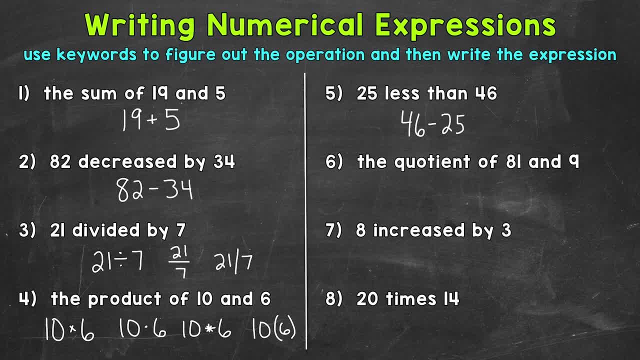 Quotient is our key word And it means the answer to a division problem. So we have eighty-one divided by nine for our numerical expression for number six, Number seven, eight, increased by three, So increased by, we are going to add three to eight.